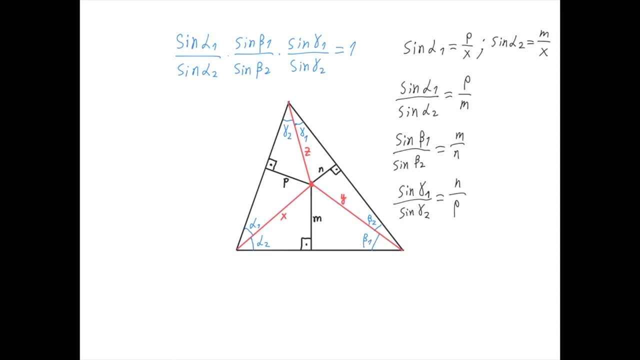 when we take the ratio of the two sines and then we get sine of beta one divided by sine of beta two is m divided by n. And in the same way we find sine of gamma one divided by sine of gamma two equals n divided by p. And these three qualities are given here. Now we just need to multiply the. 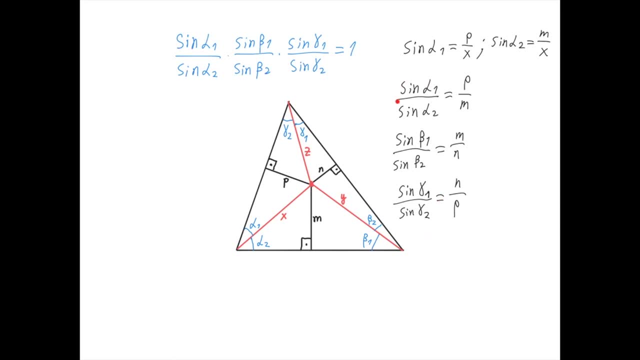 three equalities together. On the left hand side we get sine of alpha one over sine of alpha, two times sine of beta one over sine of beta, two times sine of gamma, one over sine of beta two. And on the right hand side we get the p cancels out here, the n cancels out here. 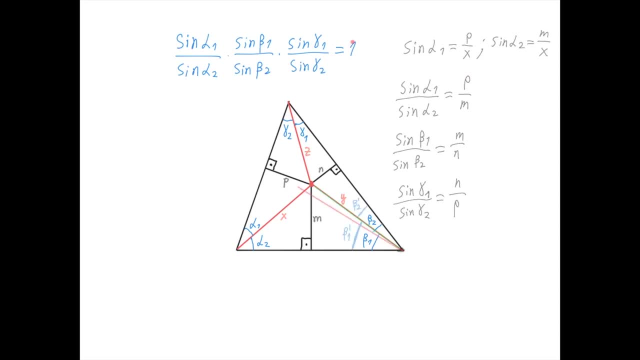 and the m cancels out here, And so the right hand side is just one. Now let's try to work in the opposite direction. Suppose that we know that this equality holds, and these angles in the equality refer to the angles alpha one and alpha two, defining this red line, the angles. 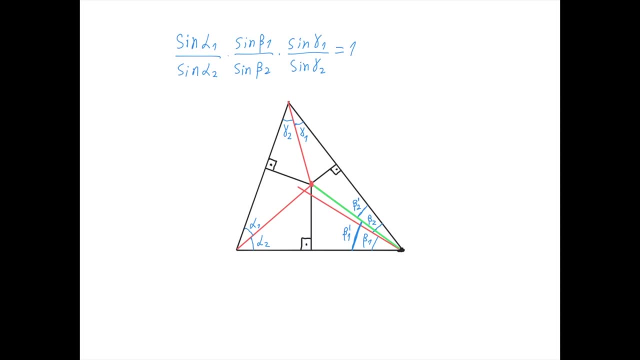 beta one and beta two defining this red line, and the angles gamma one and gamma two defining this red line. So we need to prove that the three red lines intersect at one point. So let's define this point to be the intersection of this red line and this red line, and we're going to 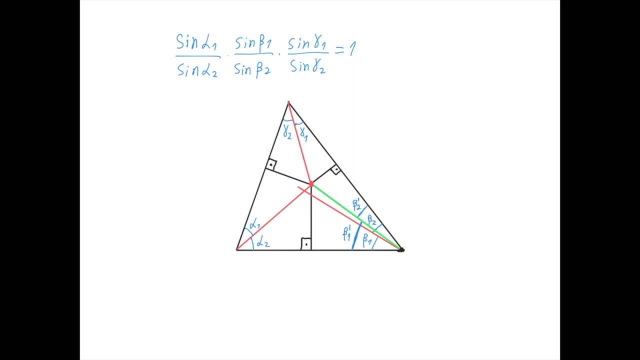 connect this point and this point with this green line. So we have to prove that the green line and this red line are actually the same line. In other words, we have to show that beta one equals beta one prime, where beta one prime is this angle defined by the green line, and we know that this 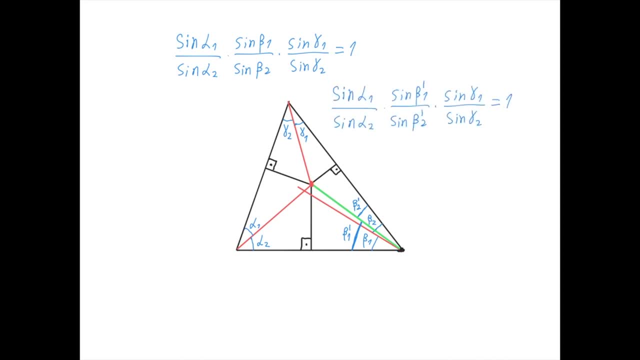 red line, this red line and this green line intersect at one point. And so we can use what we've already proved: that if we know that three lines intersect at one point, then the six angles they make with the sides of the triangle satisfy this relationship, here And now that we know that, 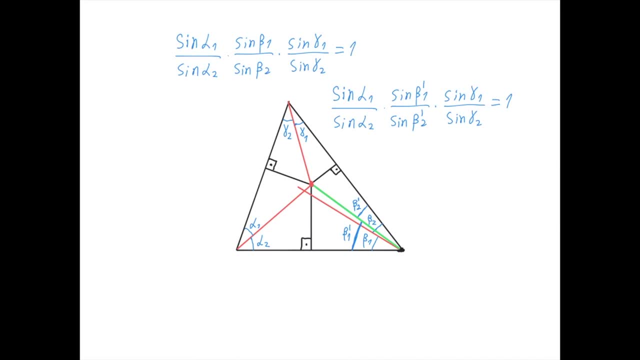 this equality holds, and this equality holds. we can divide one by the other, cancel out the alpha one, alpha two, gamma one and gamma two, and then we'll be left with sine of beta one over sine of beta two equals sine of beta one prime over sine of beta two prime. We know that the sum of beta 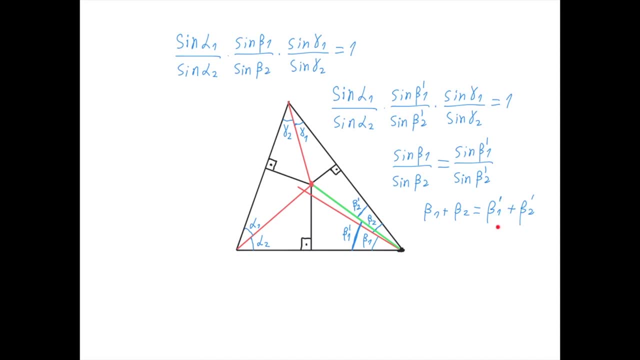 one and beta two equals the sum of beta one prime and beta two prime, because both sums equal, as you can see in the picture, this angle of the triangle. And now from this equality and to this equality, we can conclude that beta one equals beta one prime. 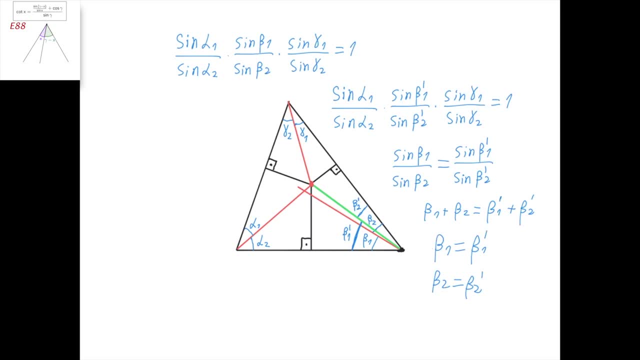 and beta two equals beta two prime, because it follows that the cotangent of beta one equals the cotangent of beta one prime and the cotangent of beta two equals the cotangent of beta two prime. And we know that beta one, beta two, beta one prime and beta two prime are between 0 and 180. 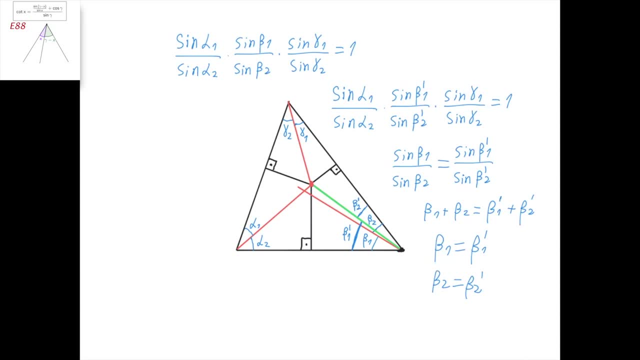 degrees and therefore beta one must equal beta one prime and beta two must equal beta two prime, meaning that the red line and the green line are actually the same line. Note that if the triangle for example here, then the solution wouldn't work quite as we described. It would still work. 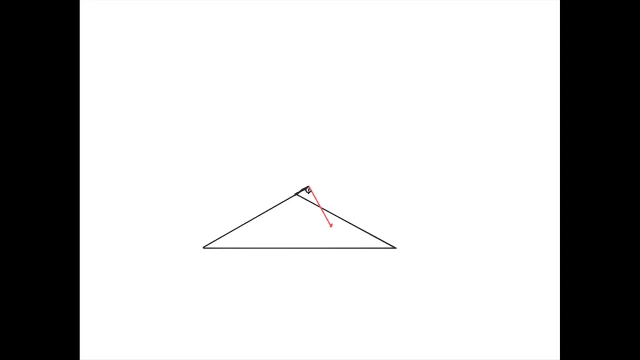 but it needs some adjustments. Instead, I'll propose a different way of proving the sine form of Chevestilram, and it would involve showing that the regular form of Chevestilram is actually equivalent to its trigonometric form or sine form. Suppose you have a triangle. 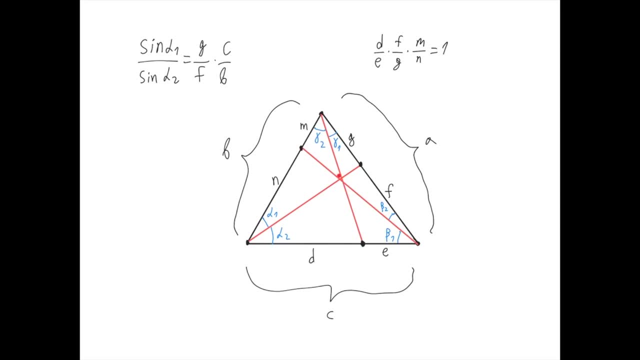 and these three lines, these two red lines. we don't know if they intersect at one point or not. What we know is that this length is d, this length is e, f, g, m and n: The sides of the triangle. 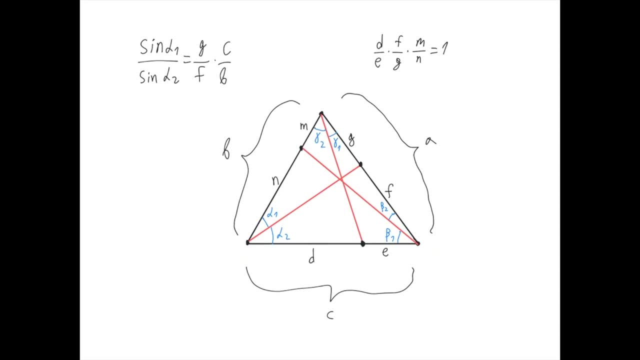 we label a, b and c and the angles, we label alpha1, alpha2,, beta1, beta2, and gamma1, gamma2.. We know that these three lines intersect at one point: if, and only if, d over e times f over g. 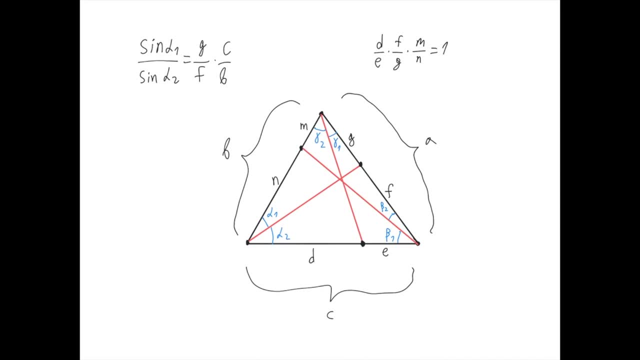 times m over n equals 1.. And we're going to prove that it is equivalent to sine of alpha1 over sine of alpha2 times sine of beta1 over sine of beta2, times sine of beta2 over sine of beta2 over sine of beta1 over sine of beta2, times sine of beta1 over sine of beta2 over sine of beta2 over sine of. 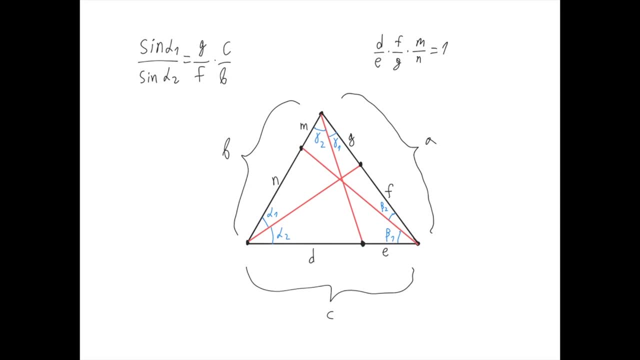 gamma1 over sine of gamma2 equals 1, which is the sine form of Chevestelram. First let's apply the law of sines for this triangle and this triangle We get that sine of alpha1 divided by sine of alpha2 equals g over f times c over b, as given here. Similarly, 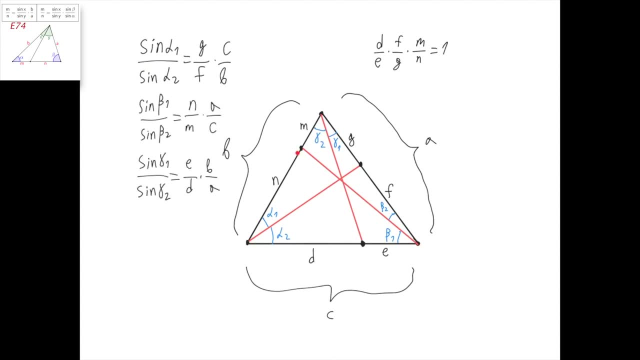 by applying the law of sines for this triangle and this triangle, we get that sine of beta1 over sine of beta2 equals n divided by m times a, divided by c over b, And sine of gamma1 over sine of gamma2 equals e over d times b over a, as given here. 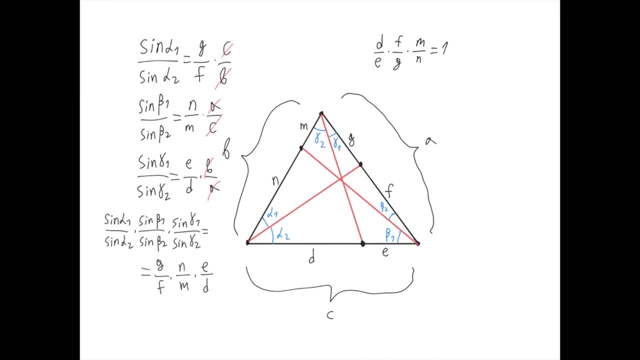 And now we can multiply these three equalities. On the left-hand side we get sine of alpha1 over sine of alpha2 times sine of beta1 over sine of beta2, times sine of gamma1 over sine of gamma2.. And on the right-hand side you can see that the sides of the triangle a, b and c cancel out here. 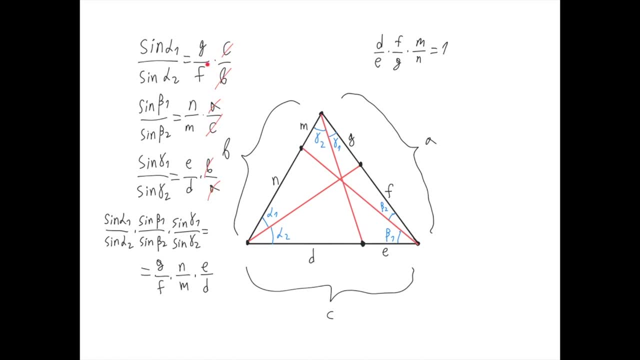 a here, b here and c here, And what is left is g over f, times n over m, times e over d. But this expression is exactly the reciprocal value of this expression, And we know that this expression equals 1 if, and only if, these three lines intersect at one point. 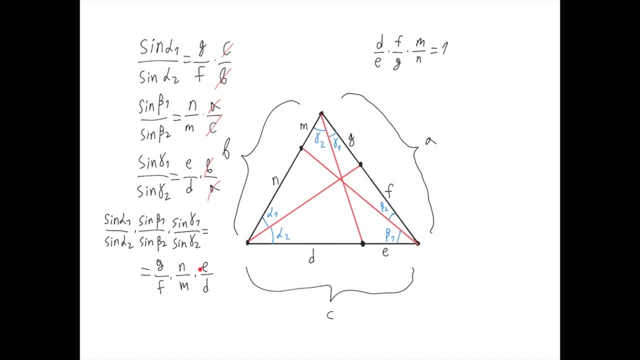 And this expression equals 1 if and only if this expression equals 1.. And since this equals this, then this expression equals 1 if and only if this expression equals 1.. But this expression to equal 1 is exactly the statement of the sine form of Cheva's theorem. 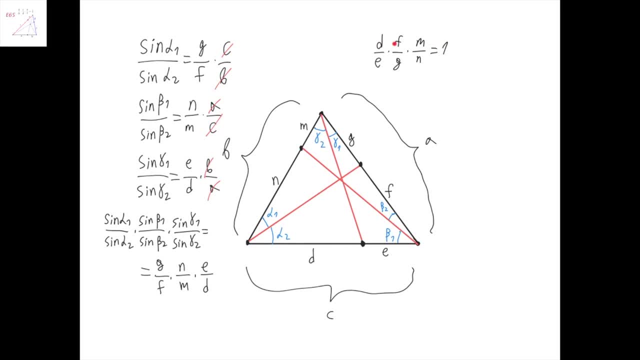 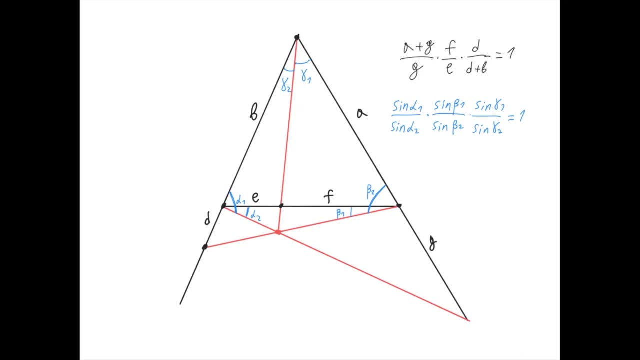 Therefore the two forms, the normal form given by this equality and the sine form given by this equality- they're exactly the same statement, so they're equivalent. Here's how the sine variant of Cheva's theorem looks like when the point is outside of the: 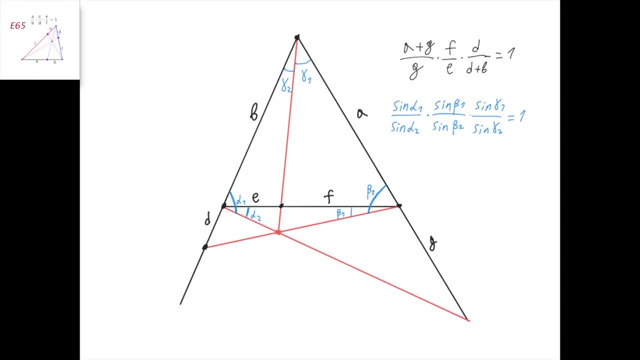 triangle In the usual form of Cheva's theorem. we know that these three lines intersect at one point: if, and only if, a plus g over g, times f over e, times d over d plus b equals 1. as given here, The trigonometric form is exactly the same. you just need to track the signs that correspond to. 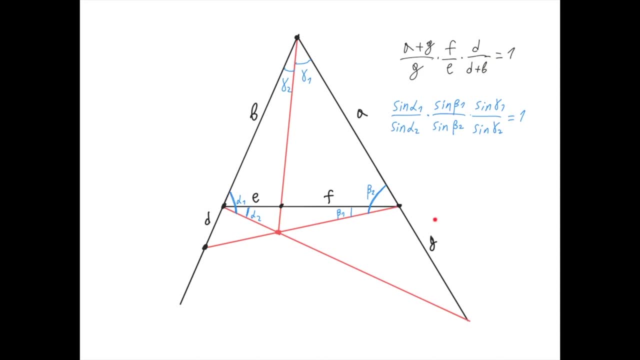 each of the segments here. For example, a plus g corresponds to the sine of alpha 1 of this angle here, and then g corresponds to this angle alpha 2.. Then f over e, f corresponds to this angle gamma 1, and e corresponds to this angle gamma 2.. And finally, d over d plus b corresponds to 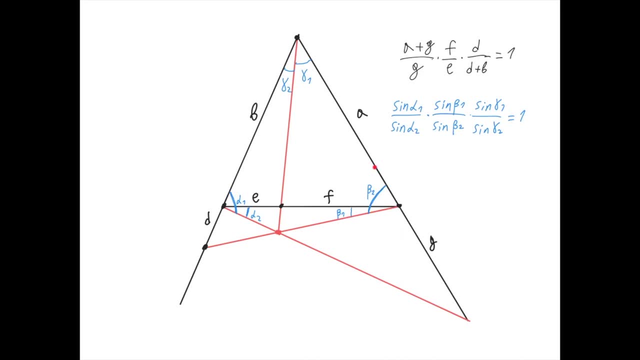 beta 1 over beta 2.. Beta 2 is the whole angle from this line to this red line. here The proof that these two are equivalent is the same. you just apply the law of signs for this triangle and this triangle, for example, and then you get that sine of beta 1. 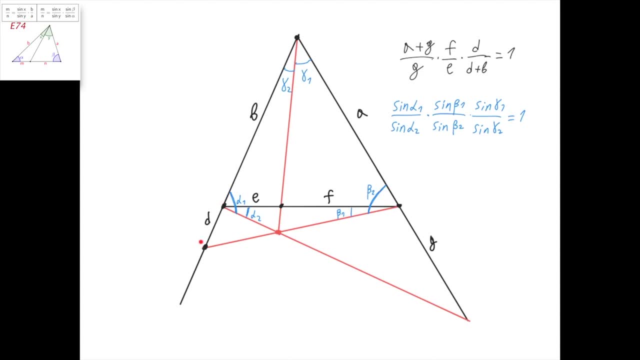 over sine of beta 2 equals d over d, plus b times a over c. if this side here is c, Then you apply the law of signs for this triangle and this triangle and you get sine of gamma 1 over sine of gamma 2 equals f over e times b over a. And finally, you apply the law of signs for 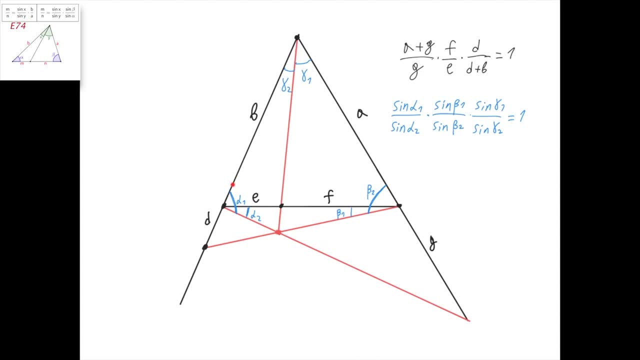 this triangle and this triangle and you get: sine of alpha 1 over sine of alpha 2 equals a plus g over g, times c over b. The a, b and c cancel out and then you get that this expression equals this expression exactly the same as in the case when this point was inside of the triangle. 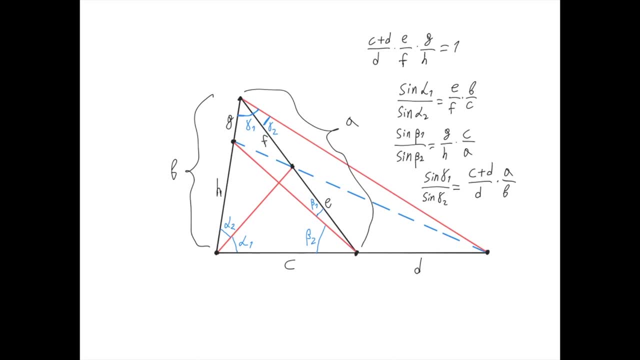 It should be noted that there exists also a sign version of Manilaus theorem. Suppose we have a triangle and three points each lying on the side of the triangle or on an extension of a side of the triangle. These three points lie on a straight line if, and only if, as you see in the 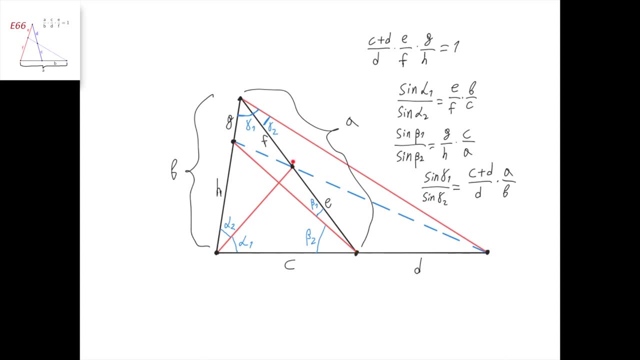 picture c plus d over d, times e over f, times g over h equals 1.. We labeled the sides of the triangle c, a and b And let's label the angles as follows: Alpha 1 here, alpha 2 here. gamma 1 here- this. 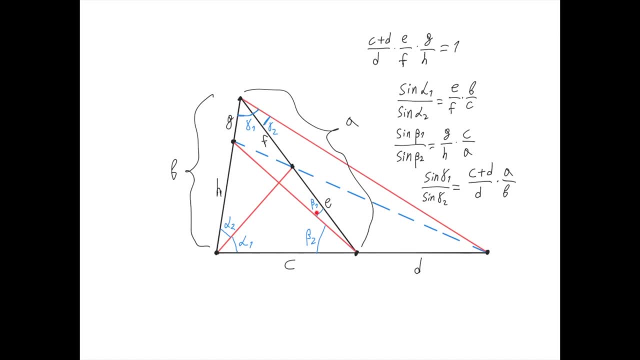 whole angle, gamma 2, this small angle, beta 1 here and beta 2 here. Then it turns out that these three particles go side by side on a straight line and then it becomes 1 cosine by sin, that's if and only if, sine of alpha 1 over sine and the potential zombies. 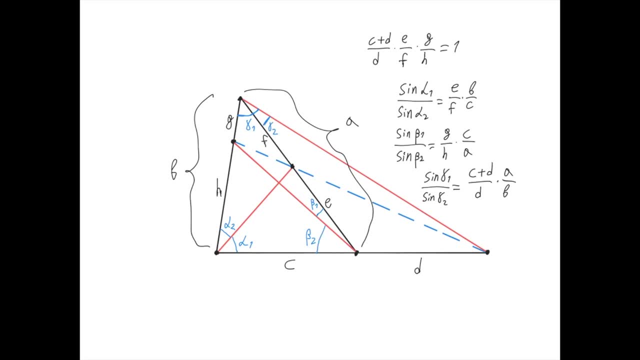 should be 1 and sine of alpha 2 by s 선생님 sigmawalia 1, bus timesших Casey false. We can prove the equivalence of these statements by just showing that sine of alpha 1 over sine of alpha 2 times, sine of beta 1 over sine of beta 2 times. 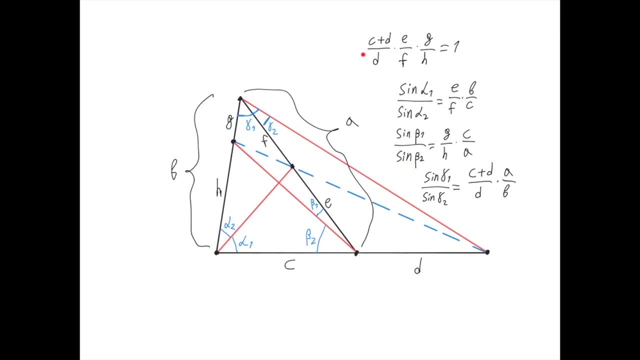 sine of gamma 1 over sine of gamma 2 equals this expression right here From the law of sines applied to this triangle. and this triangle you que That sine of alpha 1 over sine of alpha 2 equals over F times B over C, as given here. Similarly from the law of sines applied to this triangle. 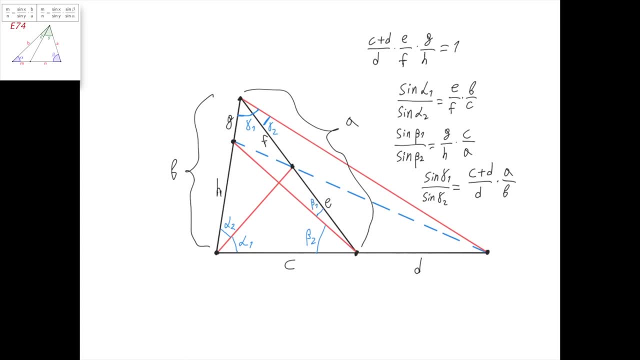 and this triangle, we get that the ratio sine beta 1 over sine of beta 2 equals G over H times C over A. given here. And lastly, by applying the law of sines to this triangle and this small triangle, we get that sine of gamma 1 over sine of gamma 2 equals C plus. 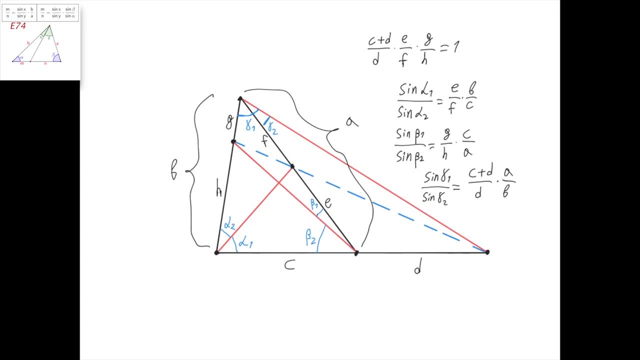 D over D times A over B, as given here. And hence, when we multiply these three qualities, on the left-hand side we get the multiplication of the ratios of sines, and on the right-hand side, the B cancels out, the A cancels out and the C cancels out, and what we have is: 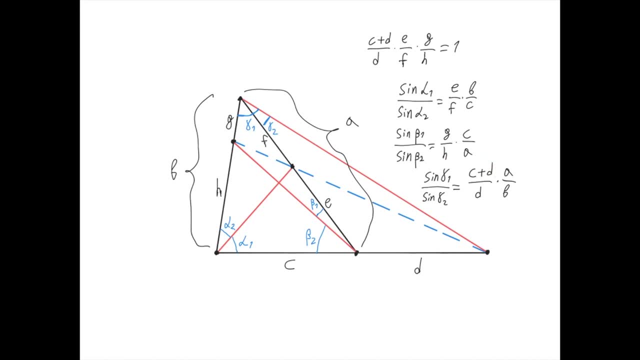 E over F, G over H and C plus D over D, which is exactly the same as this expression here, And therefore sine alpha 1 over sine alpha, 2 times sine beta 1 over sine beta 2 times sine gamma 1 over sine gamma 2 equals C plus D over D times A over B, as given here. 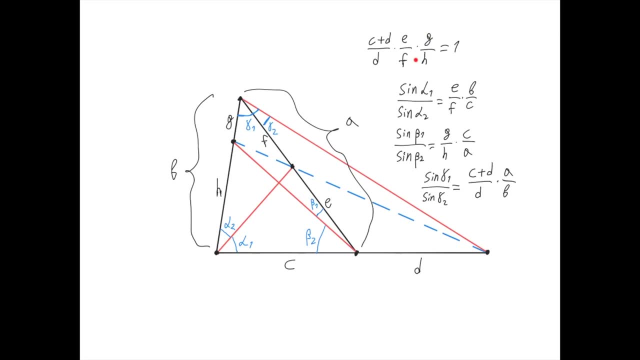 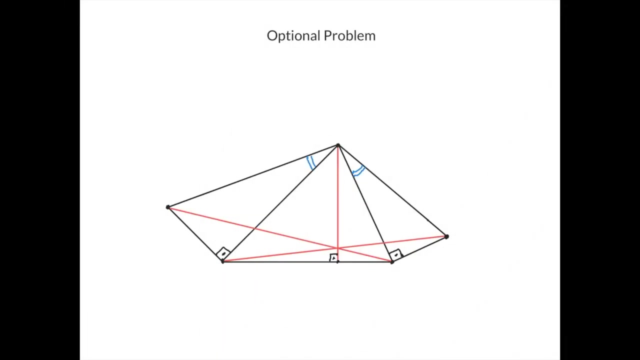 And so this expression equals 1, if, and only if, the product of these three ratios of sines equals 1, if, and only if, these three points lie on a straight line. Here's the optional problem. This is a triangle, and this here is an altitude in the triangle. 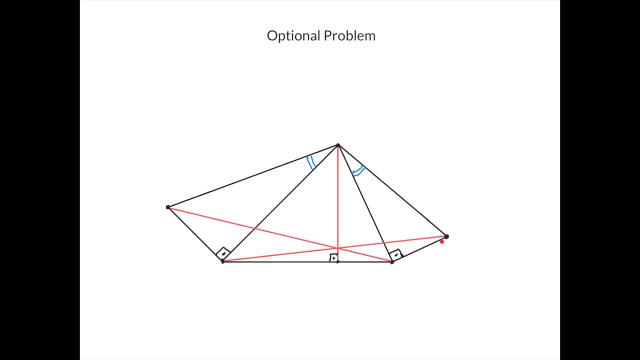 We construct this point such that this angle is a right angle- 90 degrees- and we construct this point such that this angle here is 90 degrees and such that this angle here- is this angle equals this angle. Then we connect this vertex with this point and 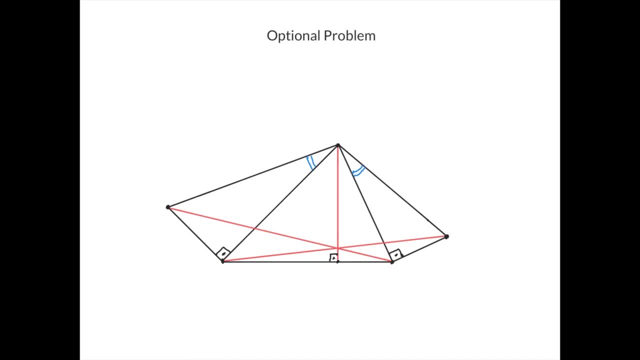 this vertex with this point, like that and like that, and we need to prove that the three red lines intersect at one point. And here's the solution. Let's label the angles in the triangle by alpha, beta and gamma. and let's label: 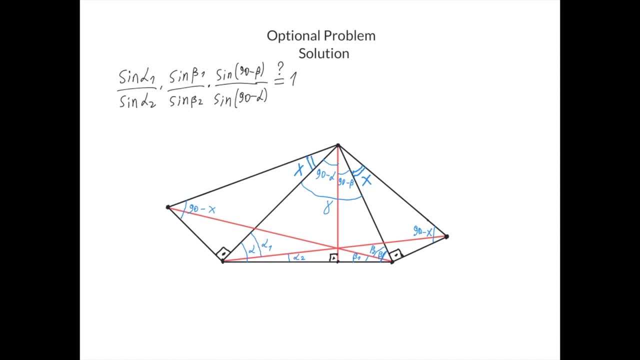 this angle here alpha 1,. this small angle here alpha 2, this angle beta 1, and this angle beta 2.. Also, let's denote this angle by X and this angle by X, and so this angle must equal 90 minus X and this angle must equal 90 minus X. Also, 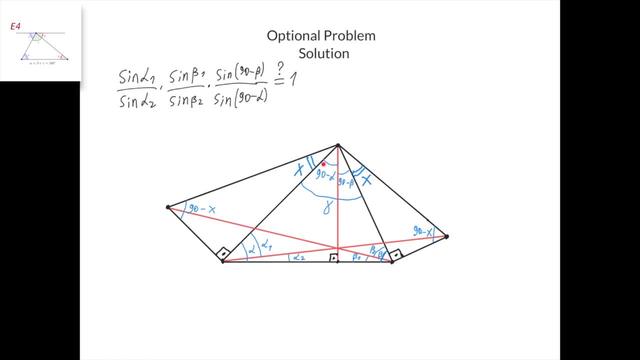 since this angle is alpha and this here is 90 degrees, we know that this is 90 minus alpha. and since this is beta, and this is 90 degrees, we have that this angle is 90 minus beta. What we need to prove is that sine of alpha 1 divided by 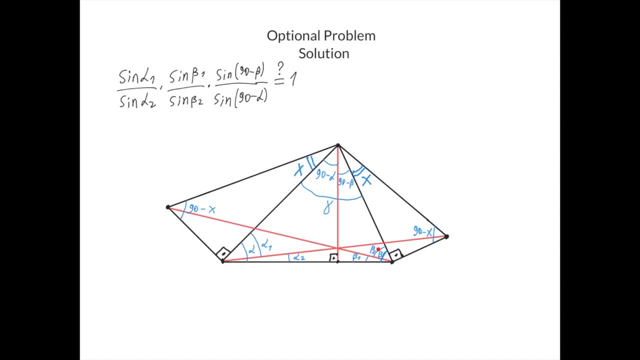 sine of alpha 2 times sine of beta. 1, divided by sine of beta 2 times sine of 90 minus beta, sine of 90 minus alpha equals 1, and the statement would follow from the trigonometric form of Chevalier's theorem. Let's denote this length. 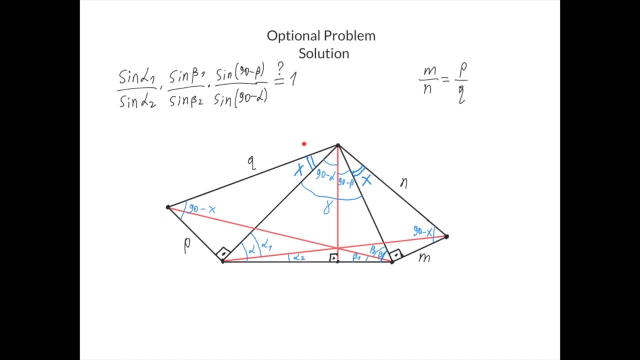 by M, this length by N, this length by P and this length by Q. Then we have similar triangles. This triangle is similar to this triangle because they have the same angles and therefore M divided by N equals P divided by Q. Now, 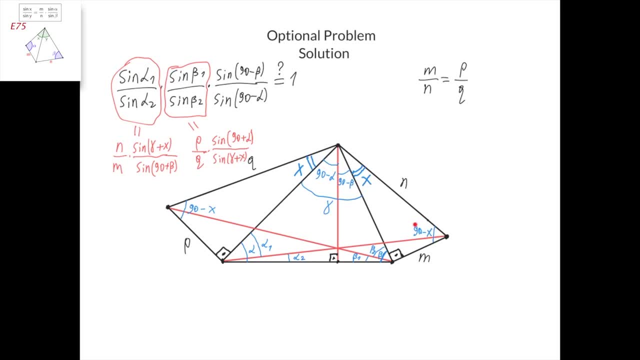 let's apply the law of sines for this triangle and this triangle, Then we get that sine of alpha 1 over sine of alpha 2 equals N divided by M times sine of gamma plus X over alpha 2.. We can apply the law of sines for this triangle and this triangle and then we 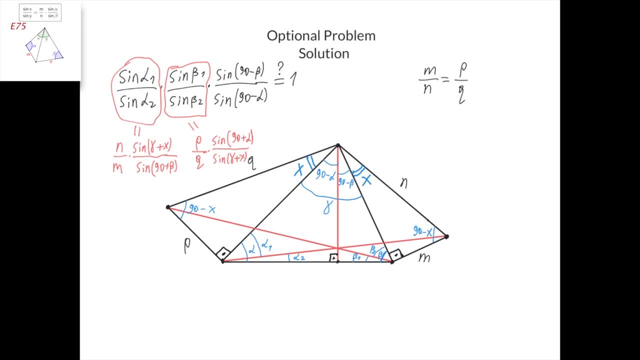 get that sine of beta 1 over sine of beta 2 equals P over Q times sine of 90 plus alpha over sine of gamma plus X, as given here. Now, because of this equality, we can cancel out N divided by M times P divided by Q. We can also cancel out sine. 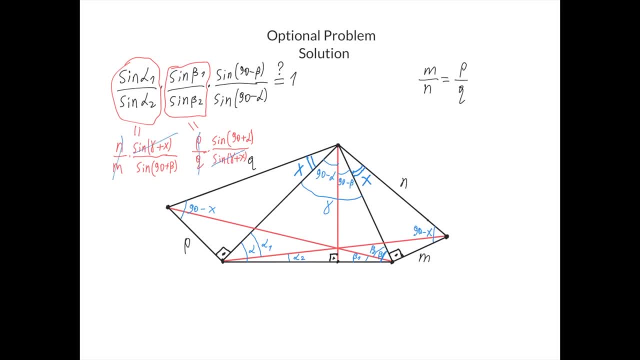 of gamma plus X over sine of gamma plus X. and now what we're left with is sine of 90 minus beta over sine of 90 plus beta, and then sine of 90 plus alpha over sine of 90 minus alpha. But we know that sine of 90 minus beta equals sine of 90 plus beta because 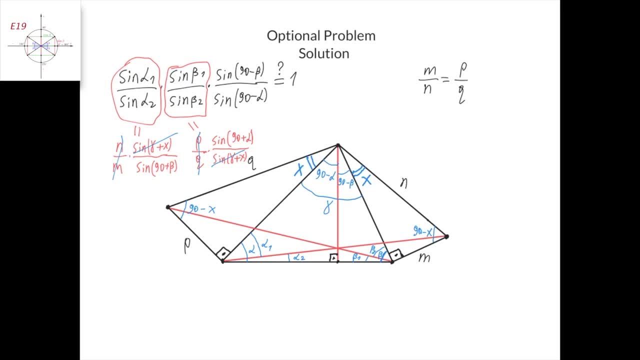 the sum of 90 minus beta and 90 plus beta is 180 degrees, so we can cancel out these two. And similarly we can cancel out sine of 90 minus alpha, which is equal to sine of 90 plus alpha, and therefore the whole expression equals 1.. Hence the trigonometric. 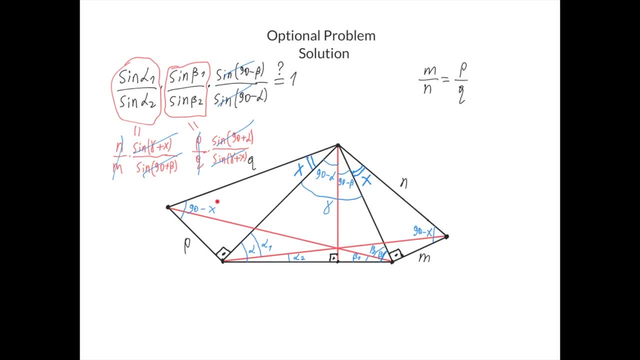 form of Cheval's theorem gives us that the three red lines intersect at one point.